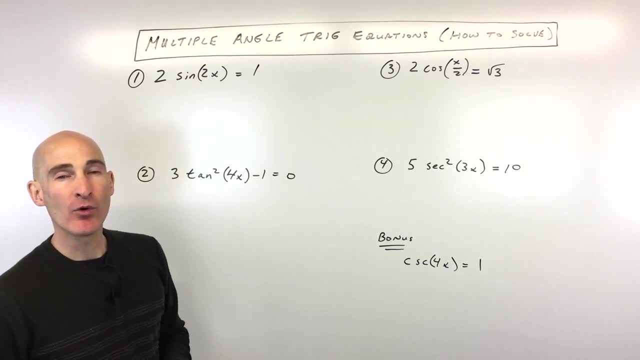 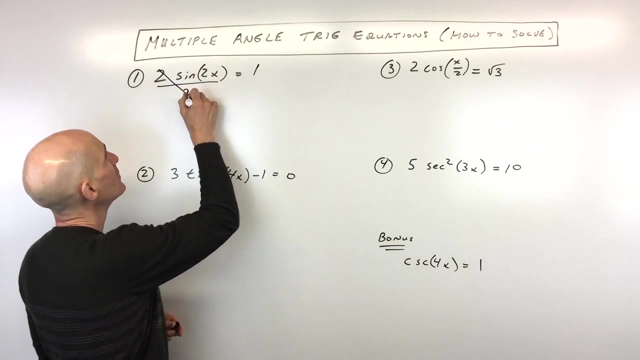 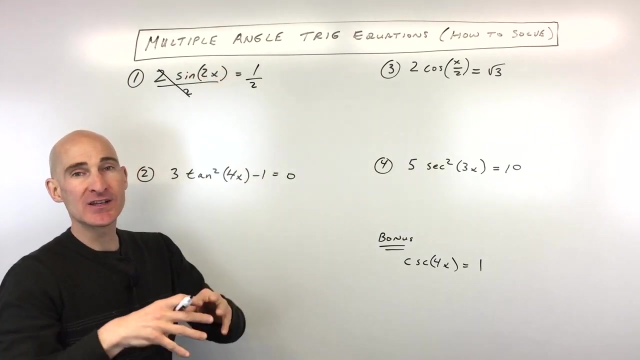 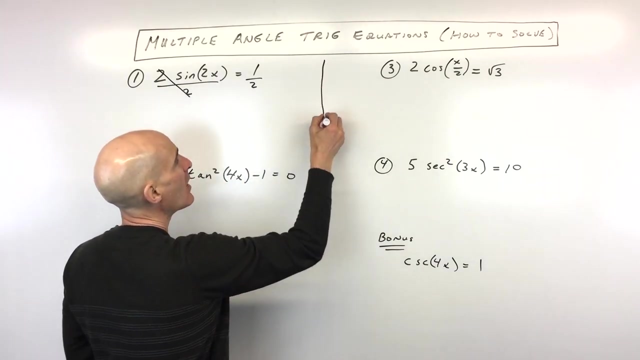 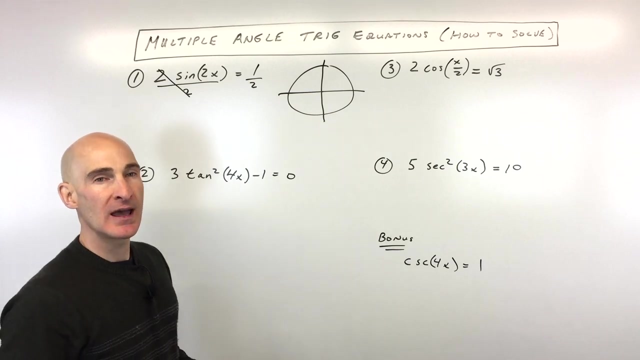 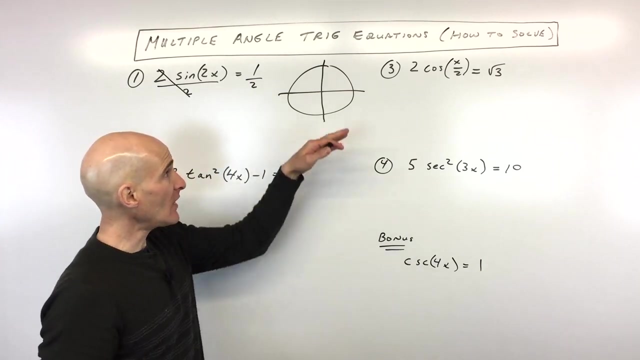 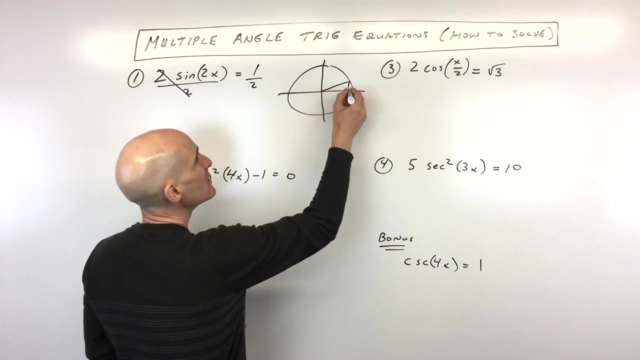 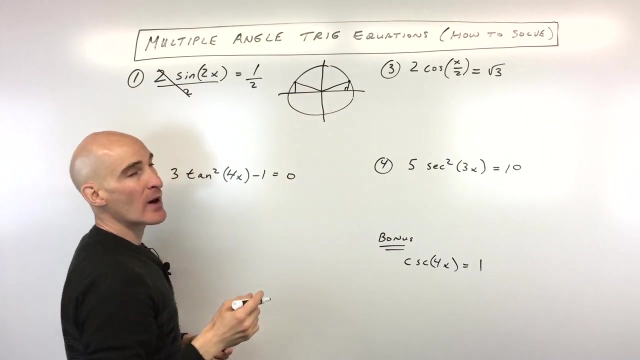 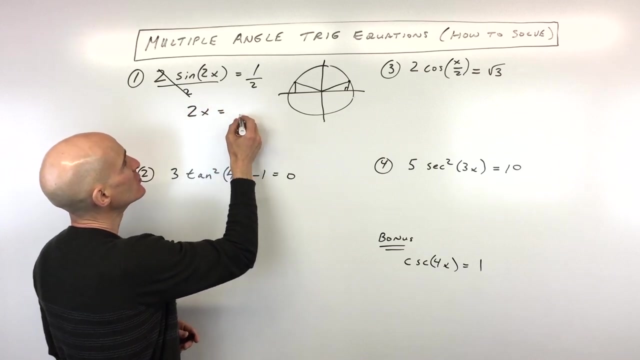 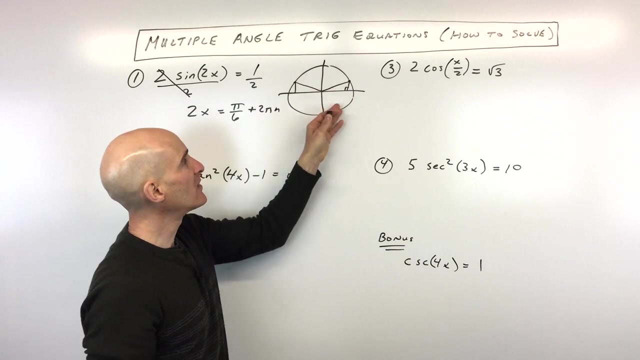 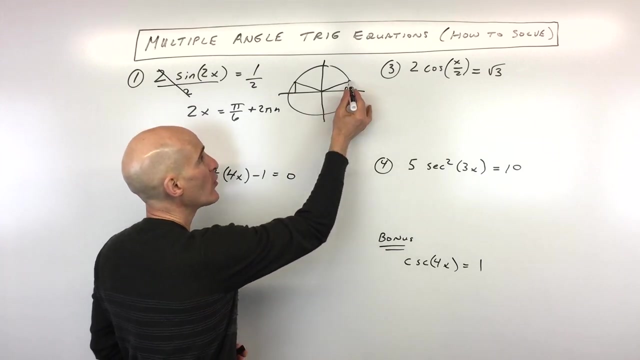 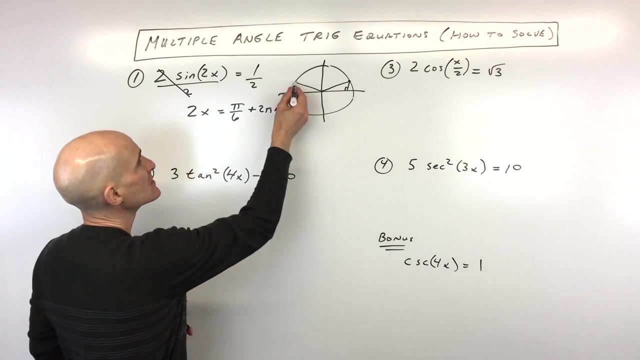 2 sine of 2x equals 1. How do we solve this problem? Well, it's just like solving an algebraic equation in the sense that what you want to do is you want to get the trig function by itself. So we're trying to get the sine of 2x by itself first. So let's go ahead and do that by dividing both sides of the equation by 2. Okay, so now we have sine of 2x equals 1 half. Now what we're going to do is we're going to treat this quantity here, this angle, as a group, as a chunk. So we're going to say sine of what angle equals 1 half. Now we're going to go to the unit circle. And if you need some help reviewing the unit circle, I'll put a link to a video I talked about how to master the unit circle and give you some practice with that. So check that video out. But we're going to jump into this. Sine of 2x equals 1 half. Now remember the sine is the y coordinate. And on the unit circle, where does the y value equal 1 half? Well, you can see that's going to be at a 30 degree reference angle. That's going to be right here. And it's also going to be in the second quadrant right here. Okay, now what we want to do, is we're going to write this as a general solution. And so what we want to do is we're going to say that 2x is equal to pi over 6, which is 30 degrees, plus 2 pi n, where n is an integer, meaning you know you can add 2 pi. That's like going once around the circle. You can add another 2 pi, another 2 pi. Or you could add like a negative 2 pi, negative 4 pi. If you keep going around 2 pi, that's one revolution. You're going to end up in the same point on the circle where the sine value, the y coordinate, is going to be equal to positive 1 half. Now also over here, this is at 150 degrees, or 5 pi over 6. So let me write that down. 2x equals 5 pi over 6, plus 2 pi n. Again, because if you add 2 pi, you go once around the circle, you end up in the same 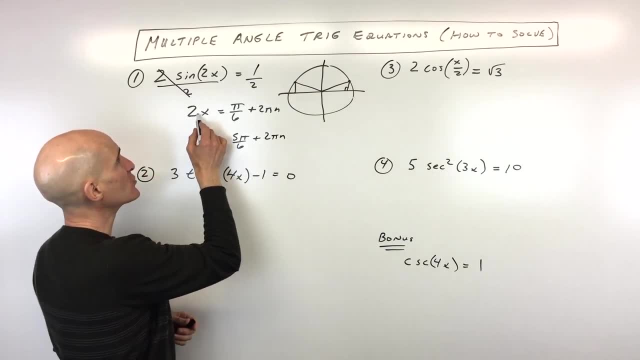 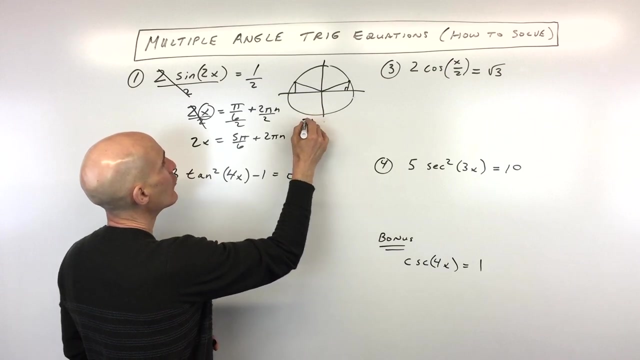 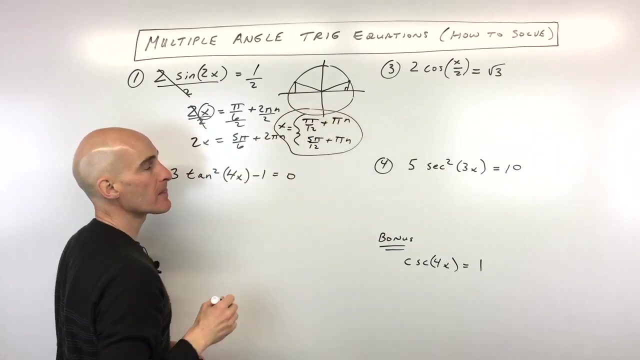 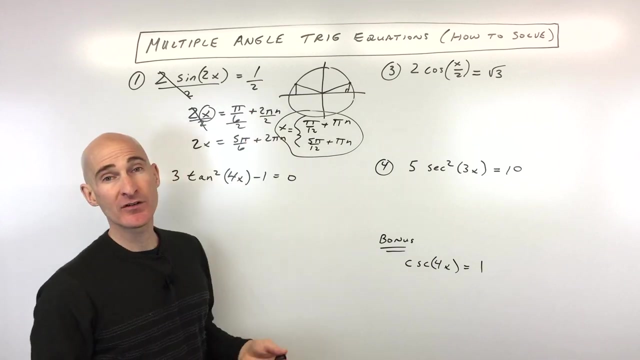 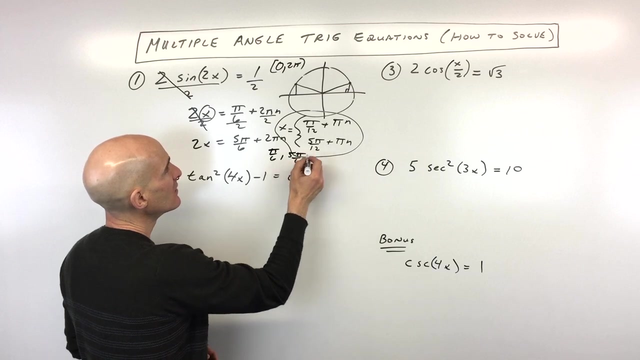 spot. You get that sine value of 1 half. But we're not interested in solving for 2x. We're actually solving for 1x. So what I'm going to do is I'm going to divide this by 2, everything on the left and right sides by 2. So if we do that, we're going to get the sine value of 1 half. So we're going to do that. So if we do that, you can see we're solving for x. But now what we're getting is we're getting pi over 12, plus pi n. And here we're getting 5 pi over 12, plus pi n. And that's our general solution for what x equals. So let me just circle that for us. Now if the instruction said, you know, not to get a general solution, but just to solve for all the angles to satisfy this equation from 0 to 2 pi. Say, for example, like this, 0 to 2 pi. So we're going to get 2 pi, including 0, but not including 2 pi. So once around the unit circle. What you would actually do is you would list the angles going around the unit circle twice. Now I'll show you why twice. Like say, for example, this here you can see is pi over 6. This over here is 5 pi over 6. This over here would be, let's see, that's 2 pi plus another pi over 6. So what's that? That's 13 pi over 6. And then over here we would have, how much would this be? This is 12 pi, 17 pi over 6, right? But the thing is, is what we actually solve for is we solve for 2x. So what we would then do is we would divide all these angles by 2. And that would 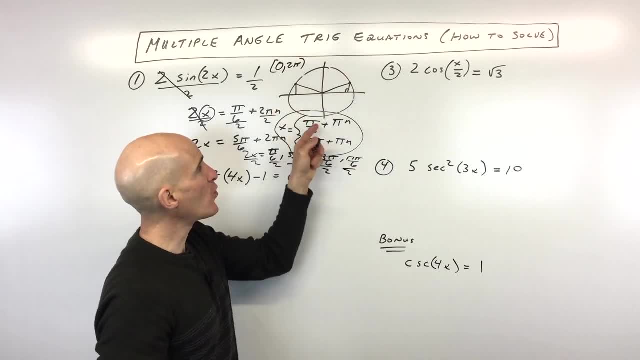 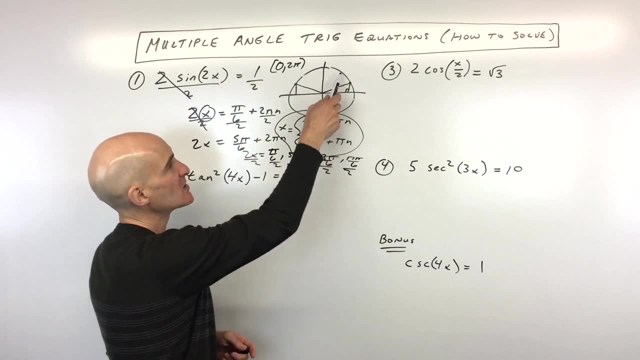 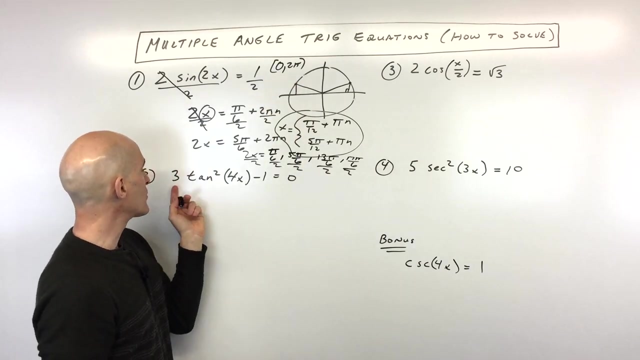 still keep you within, see, 17 pi over 12. That's still just once around the unit circle. So even though we went around twice when I found these four angles, because we actually are dividing by 2, that's going to keep us within the restricted domain here of 0 to 2 pi. So let's jump into another example so you can see how this works. So number 2, it says, 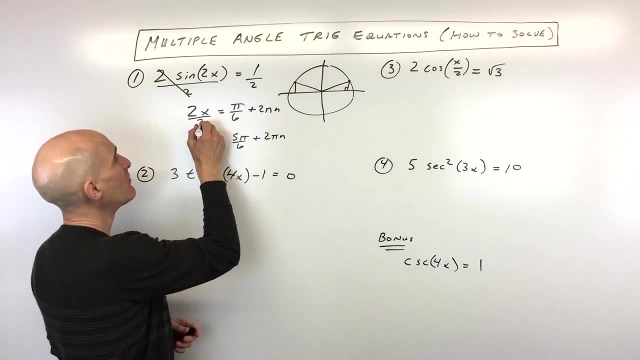 solving for 1x. So what I'm going to do is I'm going to divide this by 2, everything on the left and right sides by 2.. So if we do that, we're going to get the sine value of 1 half. So we're going to 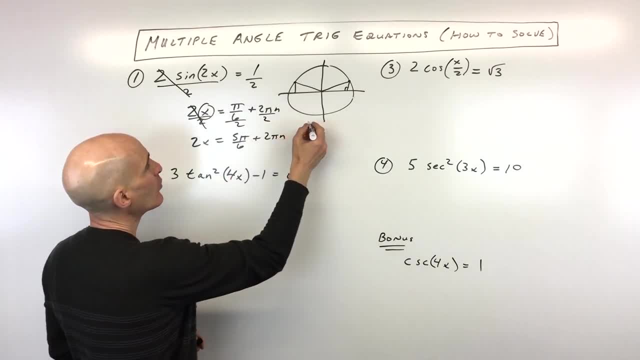 do that. So if we do that, you can see we're solving for x. But now what we're getting is we're getting pi over 12, plus pi n, And here we're getting 5 pi over 12, plus pi n, And that's. 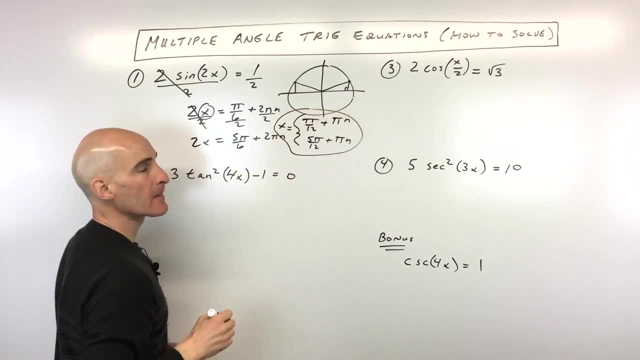 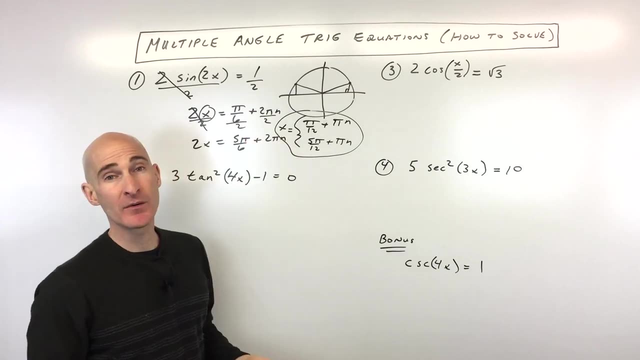 our general solution for what x equals. So let me just circle that for us Now. if the instruction said, you know, not to get a general solution, but just to solve for all the angles to satisfy this equation from 0 to 2 pi. Say, for example, like this: 0 to 2 pi. So we're going to get. 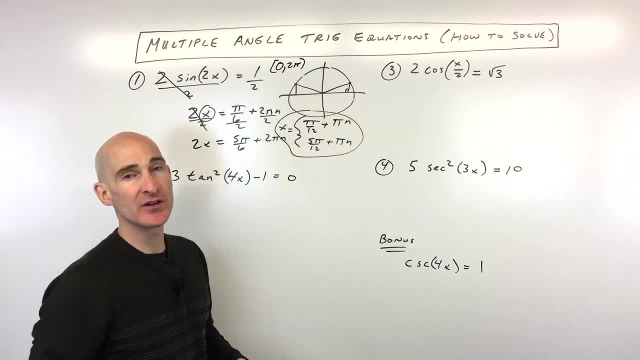 2 pi, including 0, but not including 2 pi. So, once around the unit circle, What you would actually do is you would list the angles going around the unit circle twice. Now I'll show you why twice. Like say, for example, this: here you can see is pi over 6.. This over here. 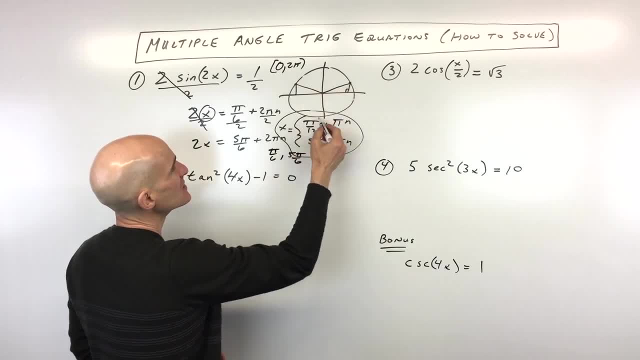 is 5 pi over 6.. This over here would be: let's see, that's 2 pi plus another pi over 6.. So what's that? That's 13 pi over 6.. And then over here we would have: how much would this be This? 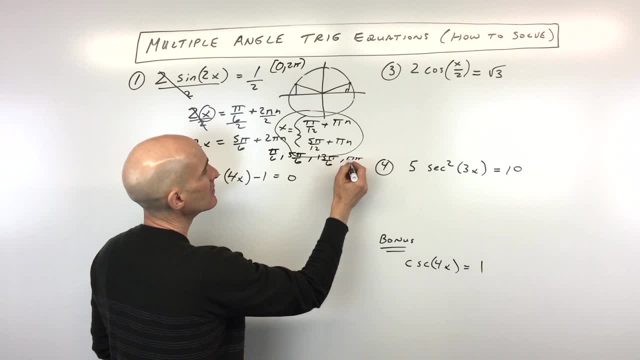 is 12 pi, 17 pi over 6, right, But the thing is, is what we actually solve for? is we solve for 2x? So what we would then do is we would divide all these angles by 2. And that would. 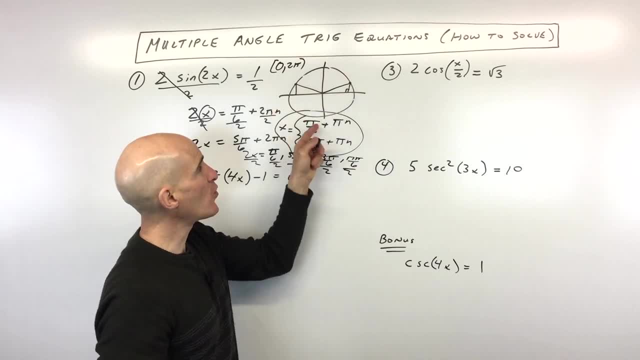 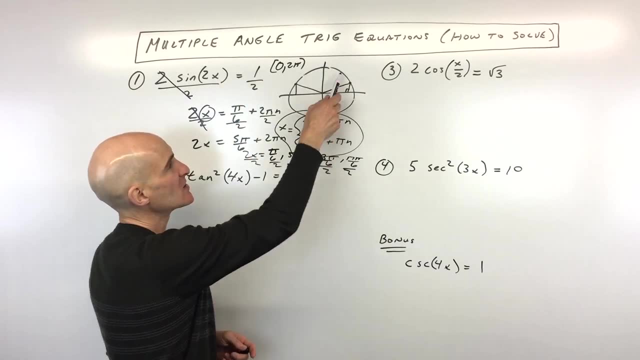 still keep you within, see 17 pi over 12.. That's still just once around the unit circle. So even though we went around twice when I found these four angles, because we actually are dividing by 2, that's going to keep us within the restricted domain here of 0 to. 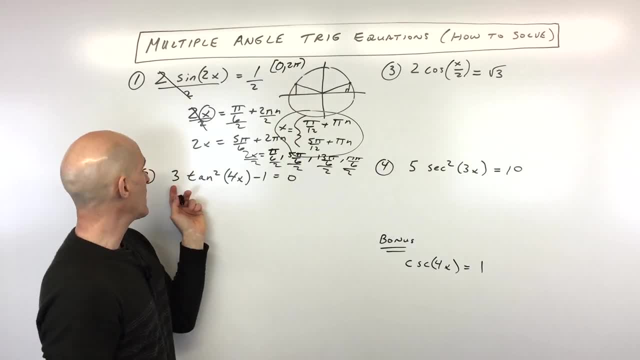 2 pi. So let's jump into another example so you can see how this works. So number 2, it says 3 tangent squared of 4x minus 1 equals 0. So, just like solving an algebra equation, we want to. 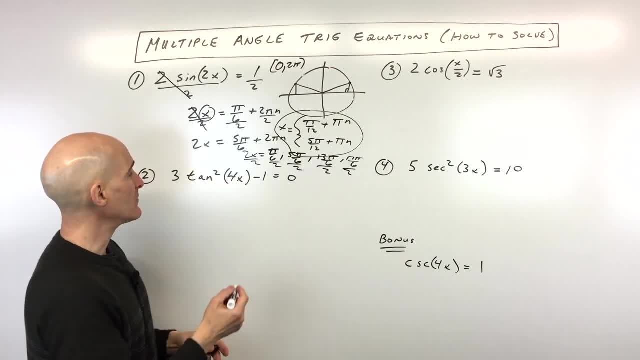 isolate that tangent. We want to get that tangent by itself. So what we're going to do is we're going to add one to both sides. OK, so we have 1.. And now we have 3 tangent squared of 4x. We're going. 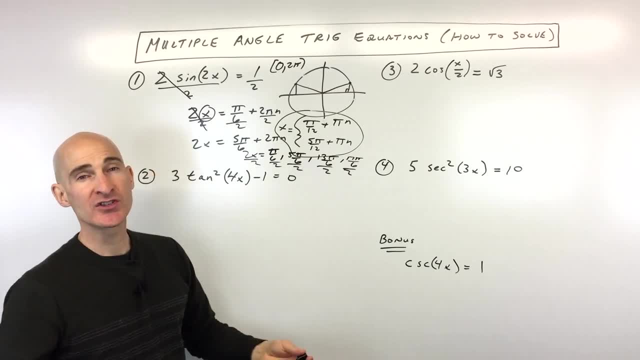 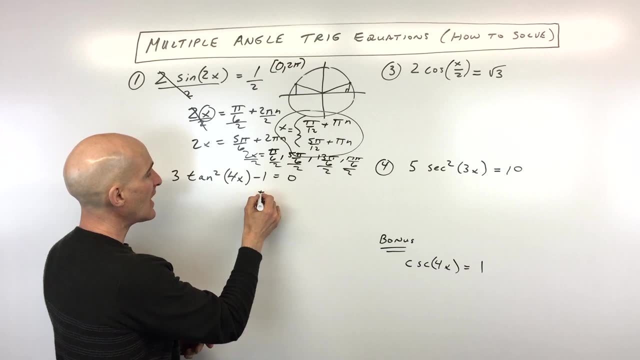 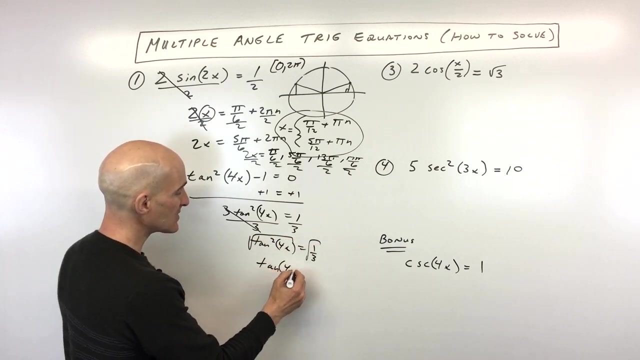 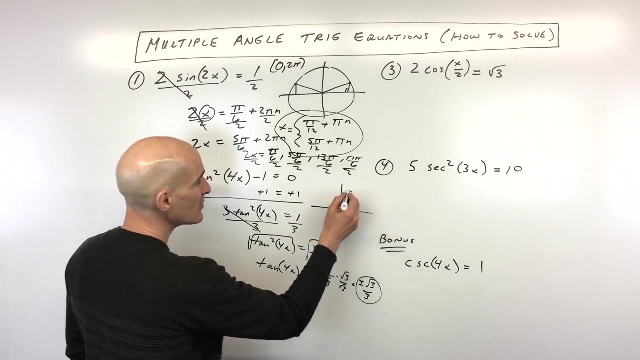 3 tangent squared of 4x minus 1 equals 0. So just like solving an algebra equation, we want to isolate that tangent. We want to get that tangent by itself. So what we're going to do is we're going to add one to both sides. OK, so we have 1. And now we have 3 tangent squared of 4x. We're going to divide both sides by 3 to get that tangent by itself. So now we're down to tangent squared of 4x equals 1 third. We're going to take the square root of both sides, because we just want to get that. So now we have tangent of 4x equals plus or minus 1 over the square root of 3, because square root of 1 is 1. Square root of 3 is square root of 3. And if we rationalize this, you can see we're getting plus or minus square root of 3 over 3. Now remember, when you take the square root of both sides, you get two answers, plus or minus. So now what we're going to do is we're going to go to the unit circle. And we're going to say to ourselves, OK, where does tangent equal square root 3 over 3? Now remember, tangent is the y value divided by the x value. 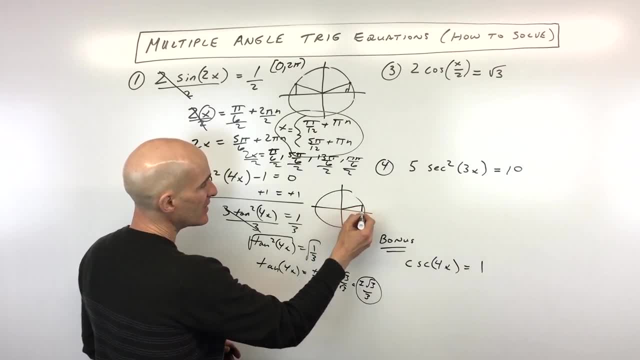 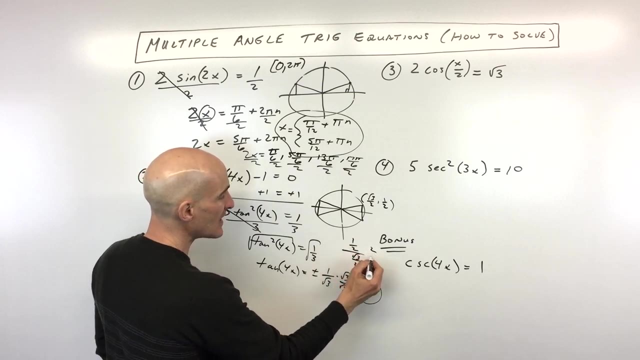 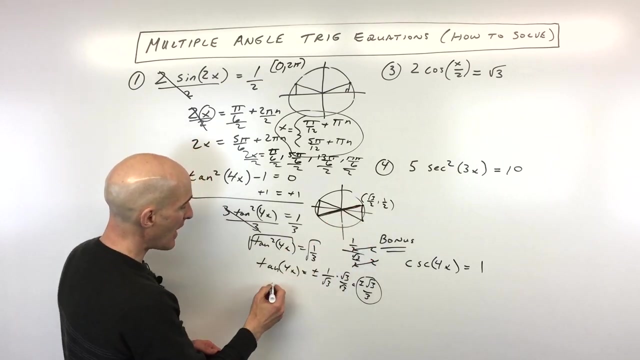 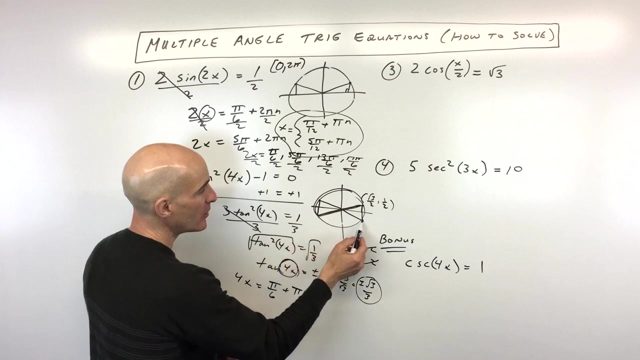 So we're going to be looking at, let's see, this is going to be right here at the 30-degree reference angles. And the reason is because, see, this point is square root 3 over 2 comma 1 half. Tangent is y over x. So you can see we're getting 1 half over square root 3 over 2. If we multiply the top and bottom by 2, see how we get 1 over square root of 3, which is what we had here? And then if you rationalize, you're going to get square root 3 over 3. But now here's the thing. If we want to write this as a general solution, what you want to do is you want to look at this. These four points. And one thing to pay attention to is that you see how these are across from each other? That's an important distinction there. So we can see this is pi over 6. OK, so 4x, we actually are solving for this angle, 4x equals pi over 6 plus pi n. Now, pi is just 180 degrees. It's just a half revolution. So every time we add pi, we end up at this point. Another pi would end up at this point, and so on. 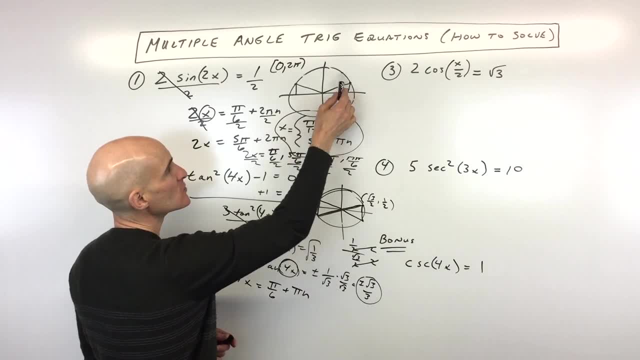 If this one, if we were to add pi, you can see that there's not a corresponding point that's 1 half revolution. 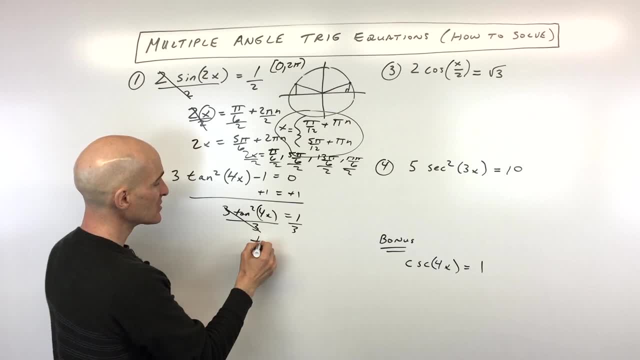 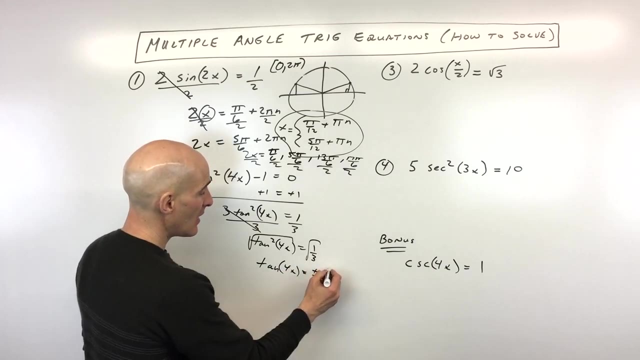 to divide both sides by 3 to get that tangent by itself. So now we're down to tangent squared of 4x equals 1. third, We're going to take the square root of both sides because we just want to get that. So now we have tangent of 4x equals plus or minus 1 over the square root of 3, because 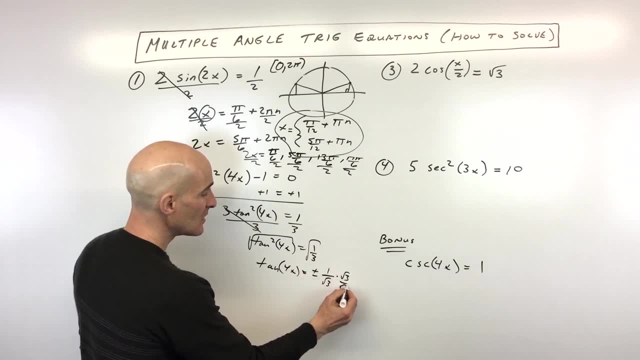 square root of 1 is 1.. Square root of 3 is square root of 3. And if we rationalize this, you can see we're getting plus or minus square root of 3 over 3.. Now remember when you take: 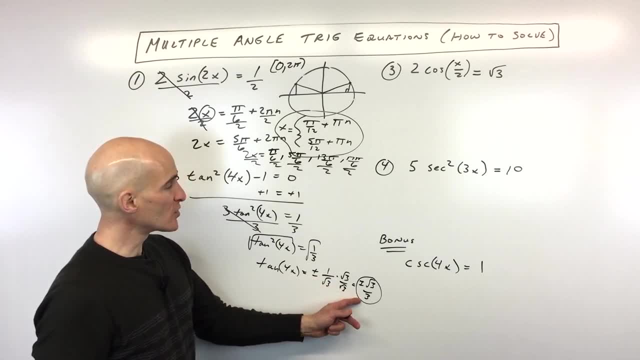 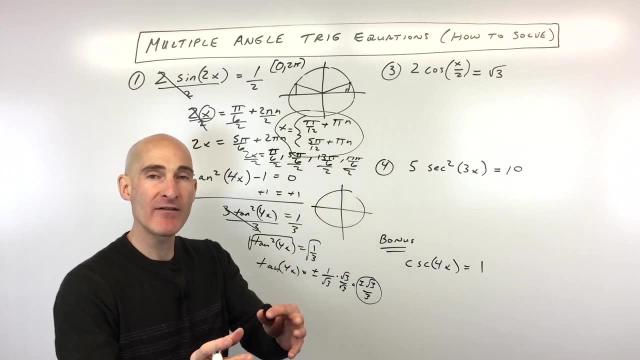 the square root of both sides. you get two answers plus or minus. So now what we're going to do is we're going to go to the unit circle And we're going to say to ourselves: OK, where does tangent equal square root 3 over 3?? Now remember, tangent is the y value. 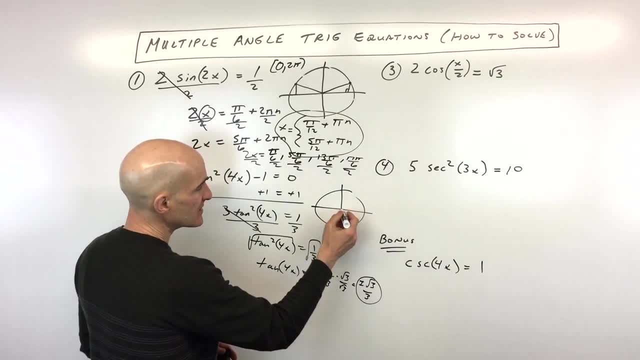 divided by the x value. So we're going to be looking at, let's see, this is going to be right here at the 30-degree reference angles And the reason is because, see, this point is square root 3 over 2 comma. 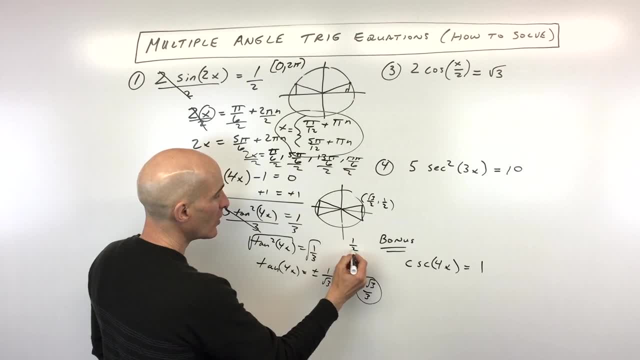 1 half Tangent is y over x, So you can see we're getting 1 half over square root, 3 over 2.. If we multiply the top and bottom by 2, see how we get 1 over square root of 3, which. 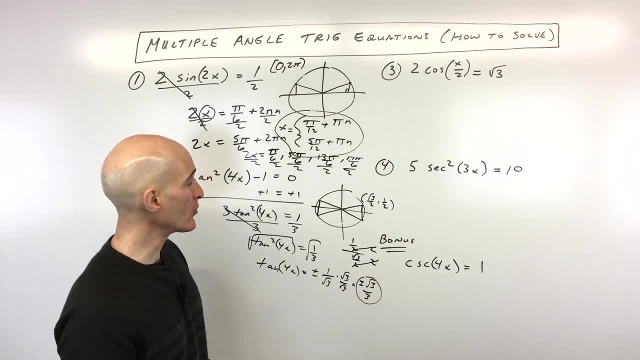 is what we had here, And then, if you rationalize, you're going to get square root 3 over 3.. But now here's the thing. If we want to write this as a general solution, what you want to do is you want to look at this. 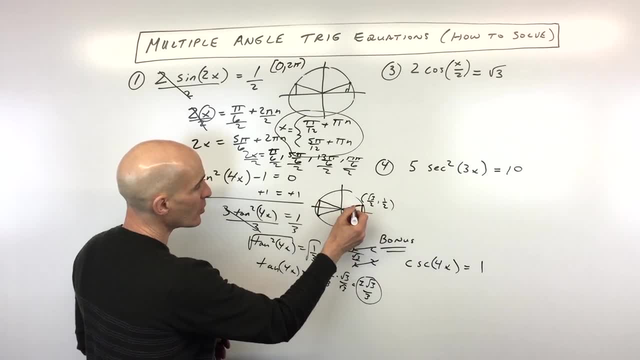 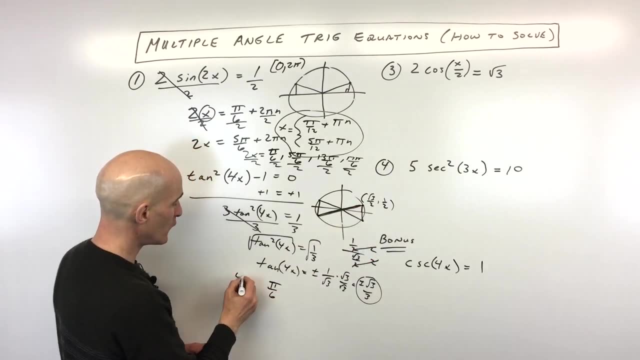 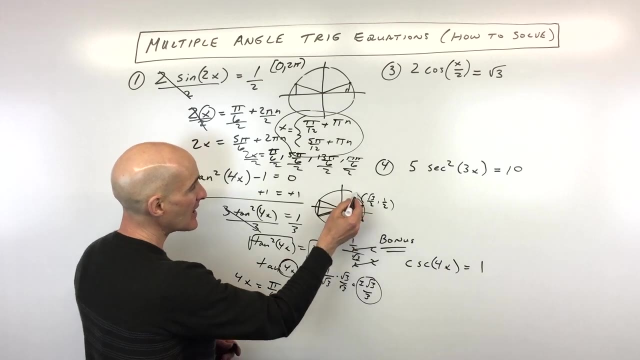 These four points, And one thing to pay attention to is that you see how these are across from each other. That's an important distinction there. So we can see this is pi over 6.. OK, so 4x. we actually are solving for this angle. 4x equals pi over 6 plus pi n. Now pi is 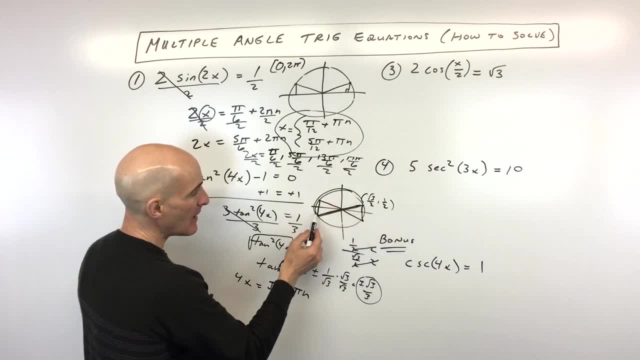 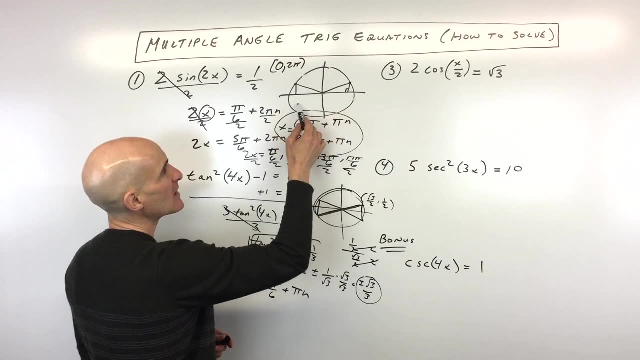 just 180 degrees, It's just a half revolution. So every time we add pi, we end up at this point. Another pi would end up at this point, and so on. If this one, if we were to add pi, you can see that there's not a corresponding point. 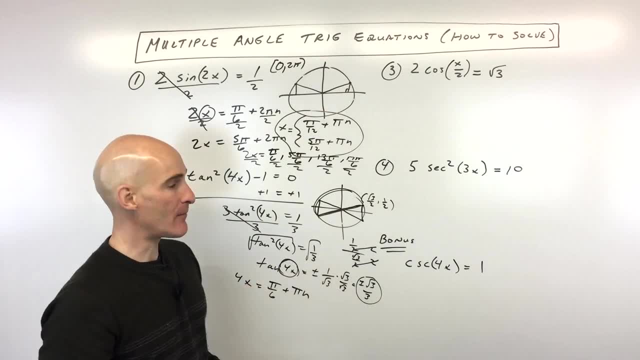 that's 1 half revolution. You know around the circle from that point. So we were having to add 2 pi, one full revolution. Here we're just adding 1 pi. So we've got 4x equals pi over 6 plus pi n, And we also 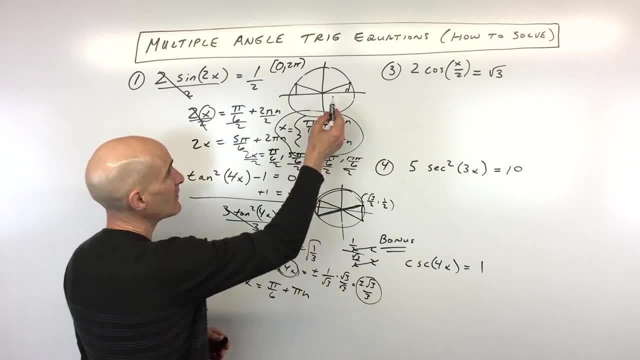 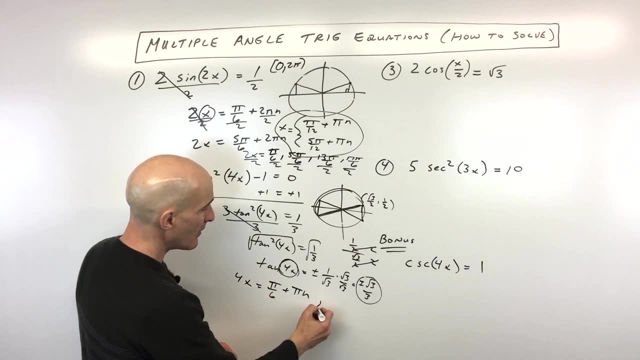 You know, around the circle from that point. So we were having to add 2 pi, one full revolution. Here we're just adding 1 pi. So we've got 4x equals pi over 6 plus pi n. And we also have 5 pi over 6 plus pi n is equal to 4x. Now, we want to just solve for 1x, so I'm 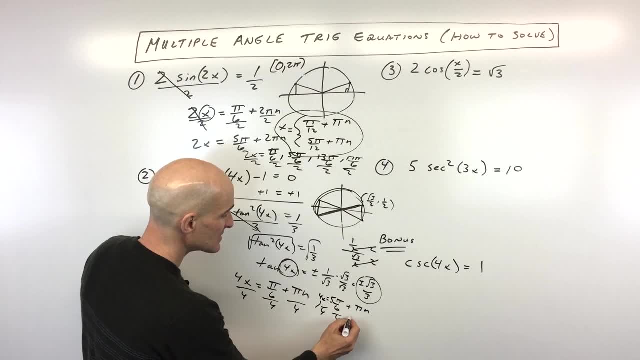 going to divide everything by 4. OK, both left and right sides. And so that comes out to what? That's pi over 24 plus pi over 4 n. 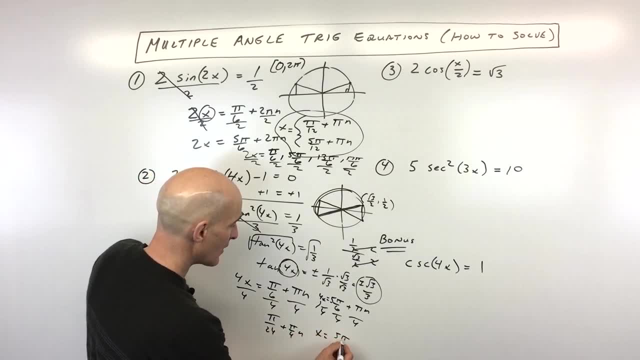 And x equals 5 pi over 24 plus pi over 4 n. So that's our general solution right there. 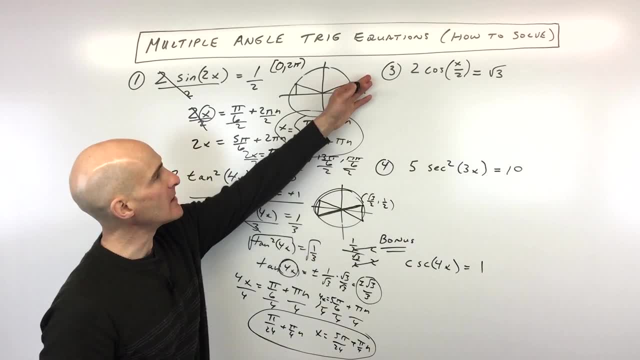 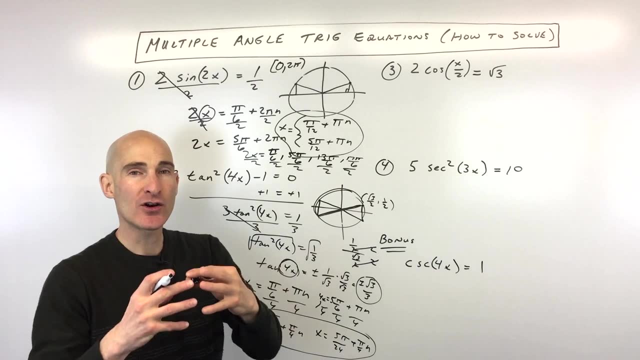 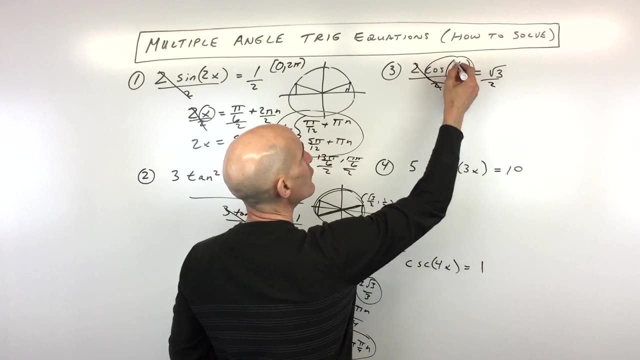 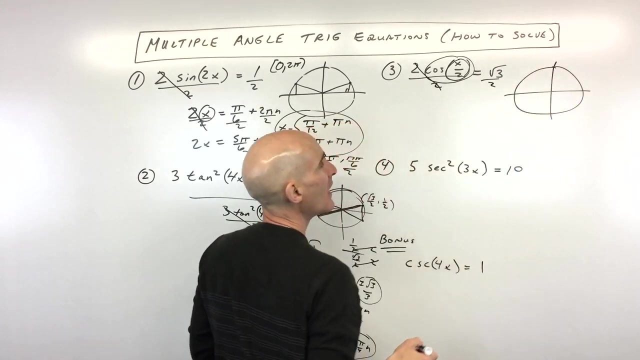 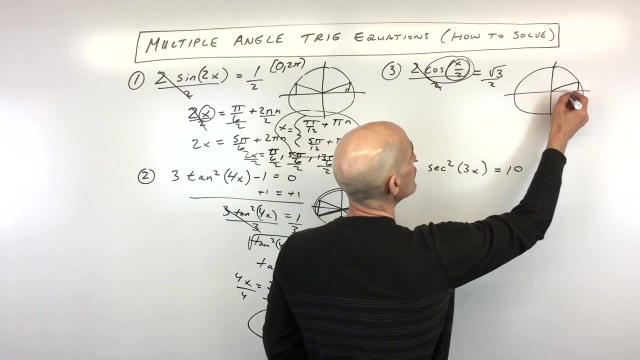 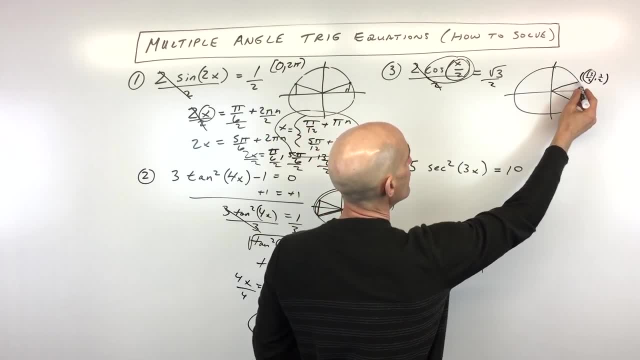 But we want to know where cosine is positive root 3 over 2, that's going to be over here at 30 degrees and over here at 330 degrees. 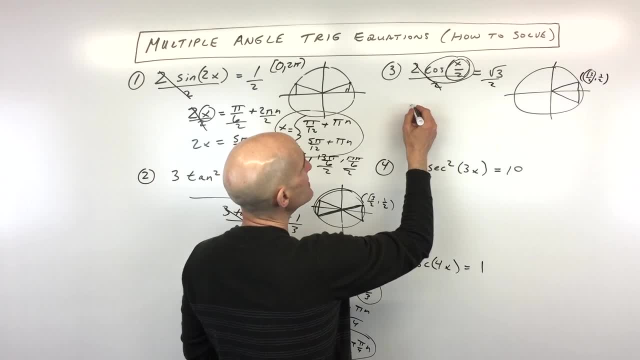 So this one I'm going to do in degrees, these ones I did in radians. So we're going to say that x over 2 equals square root 2. 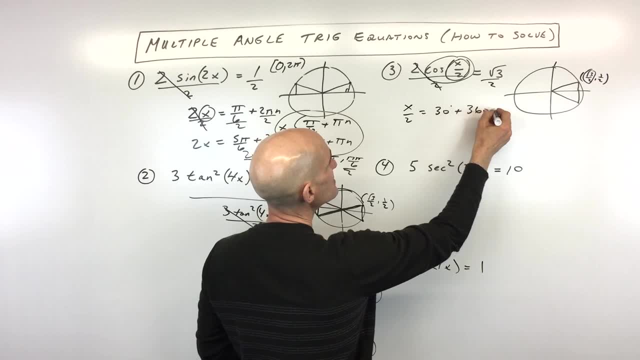 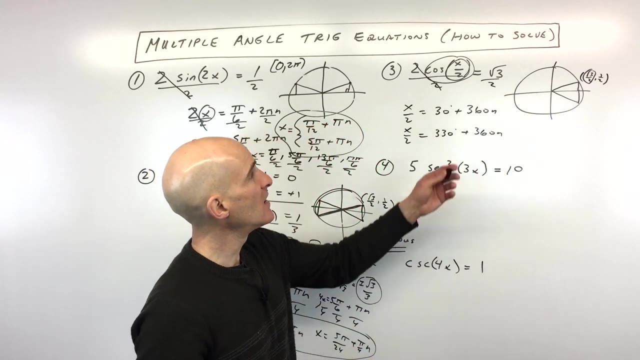 equals 30 degrees plus 360n or we could say x over 2 equals 330 degrees plus 360n now notice i'm not adding 180 degrees because that would put us over here and there's not a corresponding point where cosine equals square root 3 over 2 but now let's take it one step further let's multiply 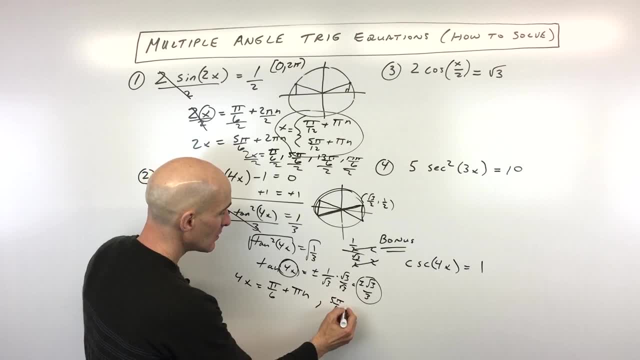 have 5 pi over 6 plus pi n is equal to 4x. Now we want to just solve for 1x, so I'm going to divide everything by 4.. OK, both left and right sides, And so that comes out. 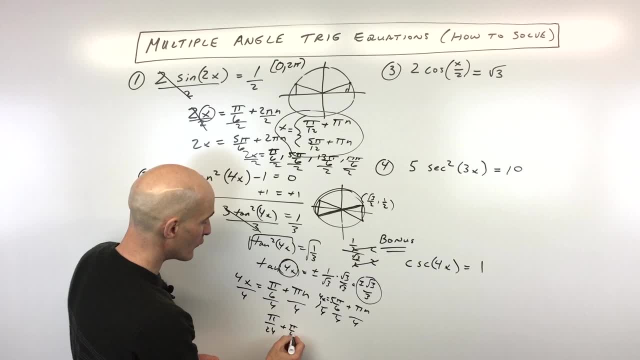 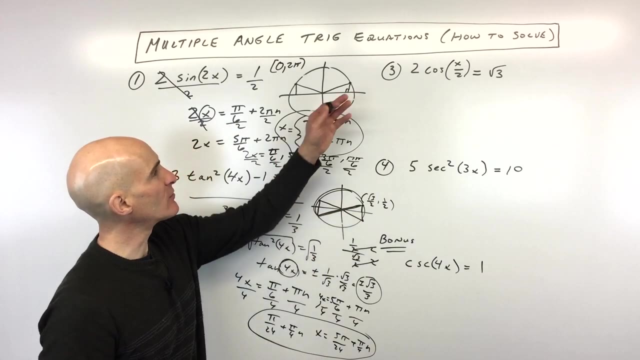 to what That's pi over 24 plus pi over 4 n, And x equals 5 pi over 24 plus pi over 4 n. So that's our general solution, right there. So that's the key. Now let's go into another example, number 3.. We've got 2 times the cosine. 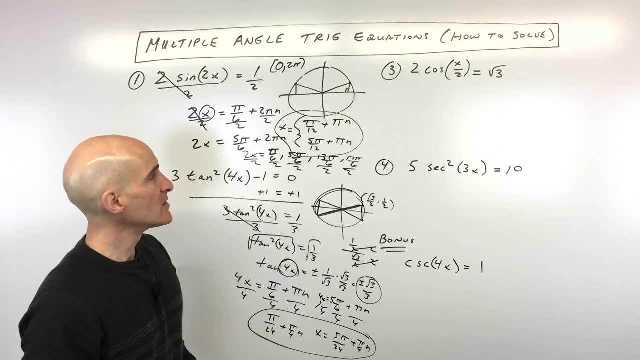 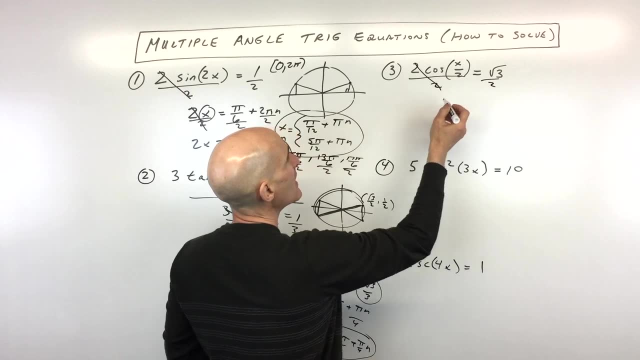 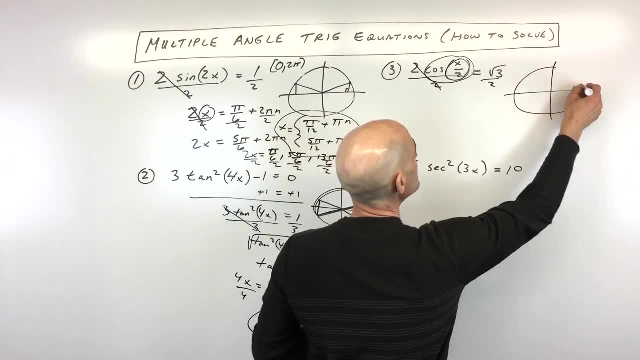 It equals square root 3 over 2.. Well, remember, cosine is the x coordinate right on the unit circle. So we're asking ourselves where's the cosine root 3 over 2.. That's again going to be at a 30-degree reference angle. See how this is: root 3 over 2, 1: 1 half Cosine. 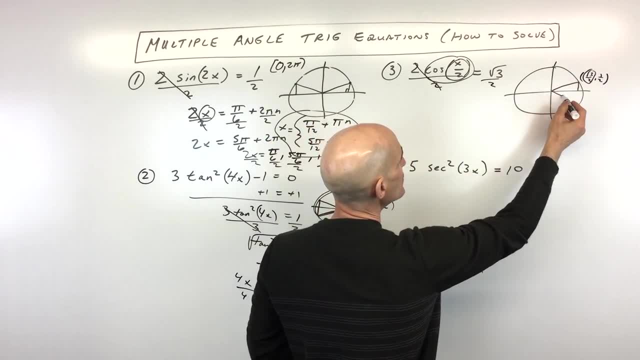 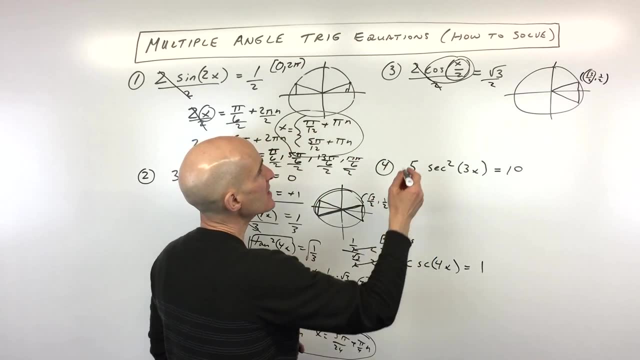 is the x, But we want to know where cosine is positive root 3 over 2.. That's going to be over here at 30 degrees and over here at 330 degrees. So this is what I'm going to do in degrees, These ones that I did in radians. 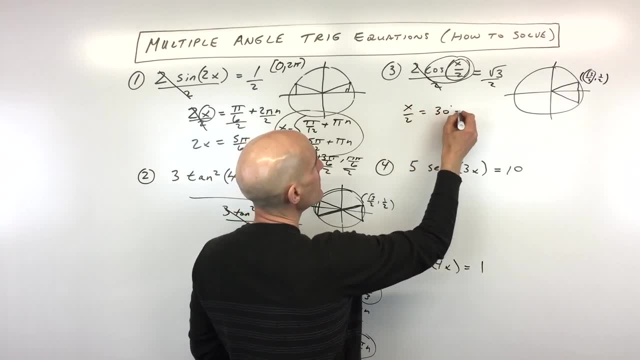 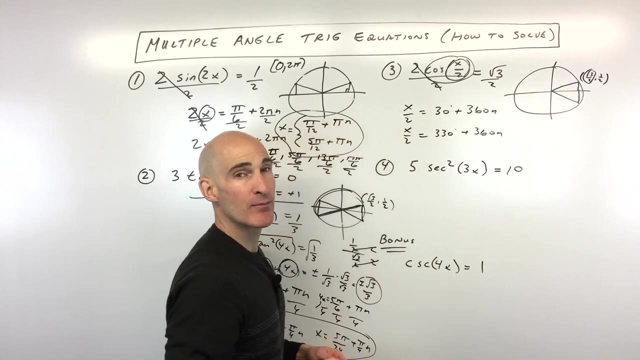 So we're going to say that x over 2 equals 30 degrees plus 360n. or we could say x over 2 equals 330 degrees plus 360n. now notice i'm not adding 180 degrees, because that would put us over here and there's not a corresponding point. 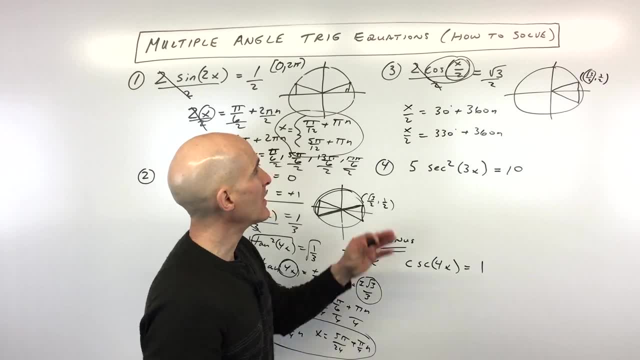 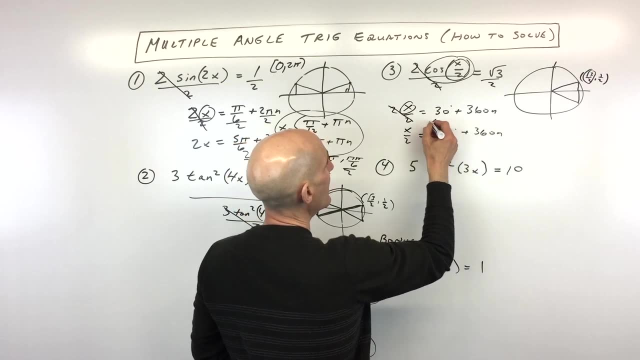 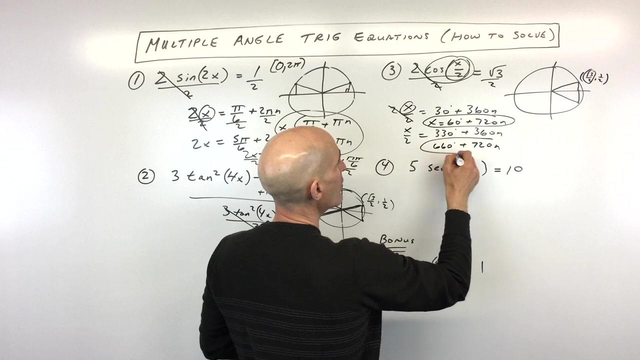 where cosine equals square root, 3 over 2. but now let's take it one step further. let's multiply both sides by 2 to get x by itself. okay. so if we do that, we're going to get x equals 60 degrees plus 720n. and if we multiply this side by 2, we're going to get 660 degrees plus 720n. okay, now if 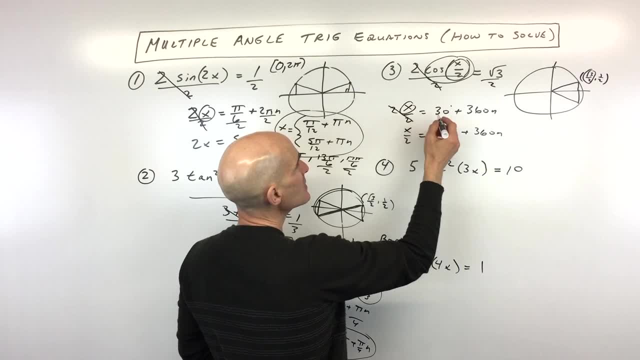 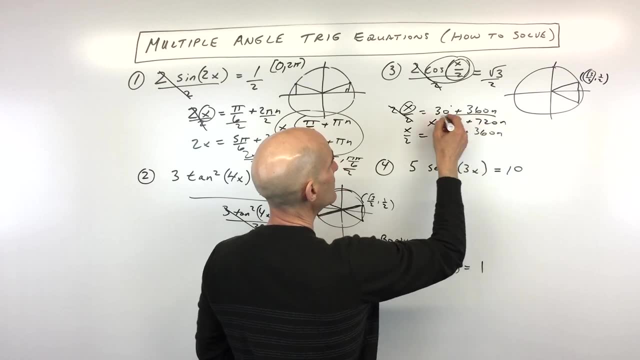 both sides by 2 to get x by itself okay so if we do that we're going to get x equals 60 degrees plus 720n and if we multiply this side by 2 we're going to get 660 degrees plus 720n okay now if 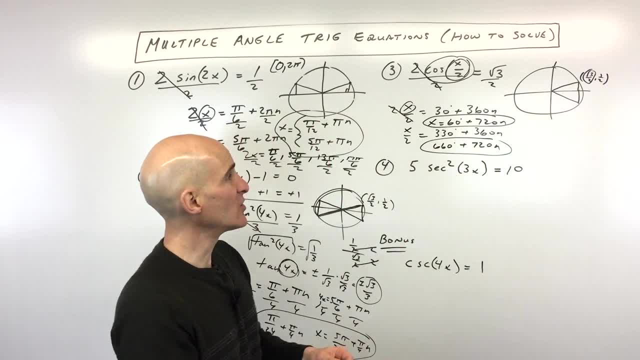 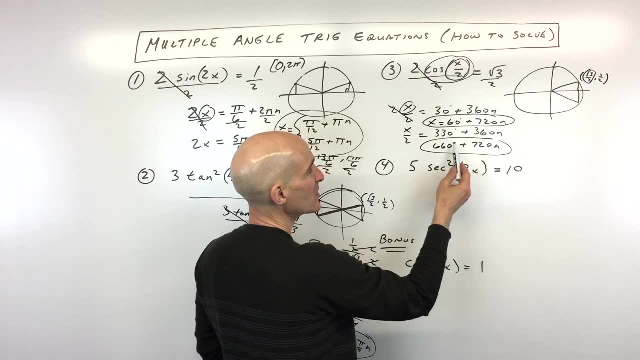 they just said, find all the solutions from 0 to 360, meaning, you know, once around the unit circle, here, if we let n equals 0, you can see we're getting x equals 60 degrees. here, if we let n equals 0, we're going to be getting 660 degrees, which is not in a restricted domain of 0 to 360. 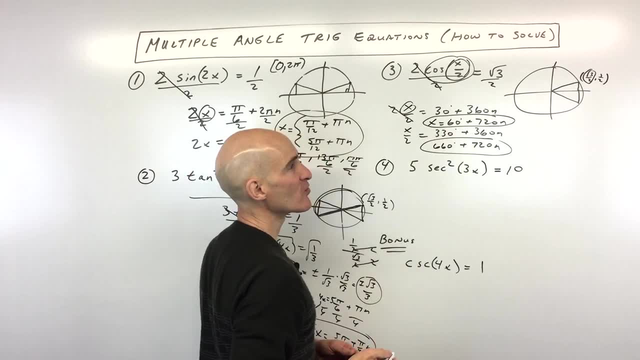 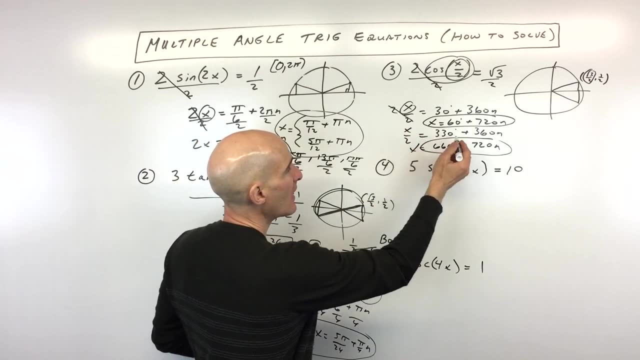 right. so you would only just get one solution here, just 60 degrees, if that was the restricted domain. but here, if we're writing this as a general solution, you know we can just have it written as 60 plus 720n or 660 plus 720n. 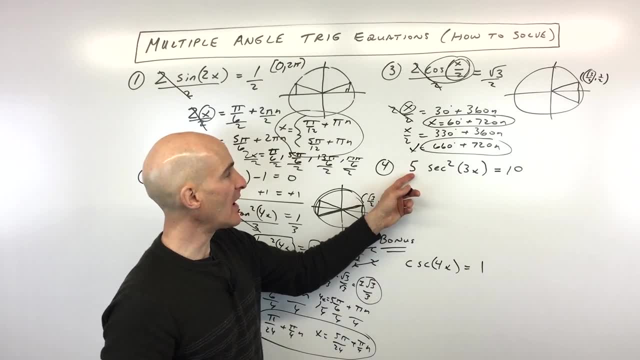 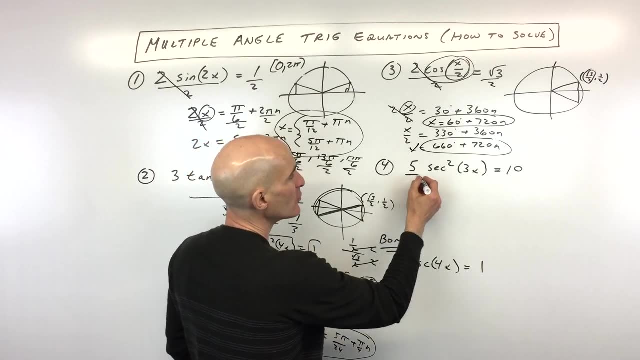 okay, let's go on to a fourth example here now. so number four: we've got 5 secant. squared of 3x equals 10, so hmm. so how are we going to solve the same idea? we're going to divide both sides by 5. 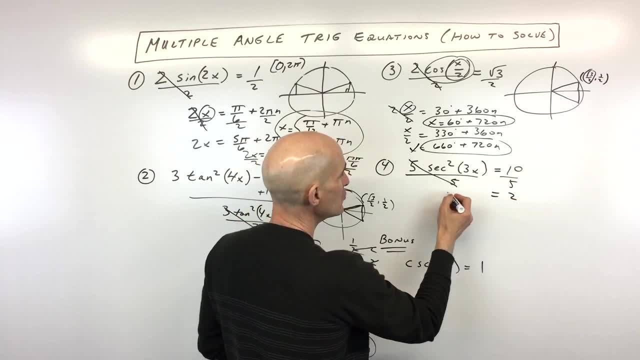 we're trying to get that secant by itself, so that comes out to 2. so we're saying secant squared of 3x is equal to 2.. secant, though, is really what it's. the reciprocal of cosine 2 is like 2 over 1, but now what i'm going to do is i'm going to take the reciprocal. 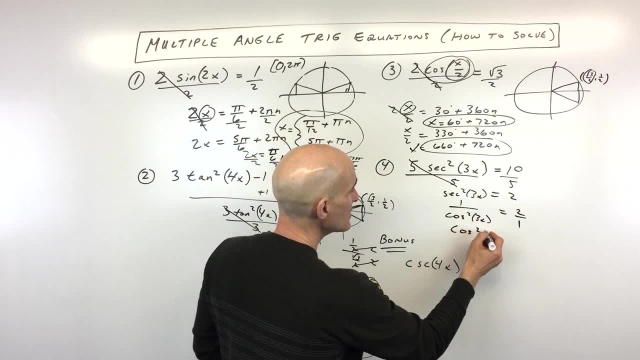 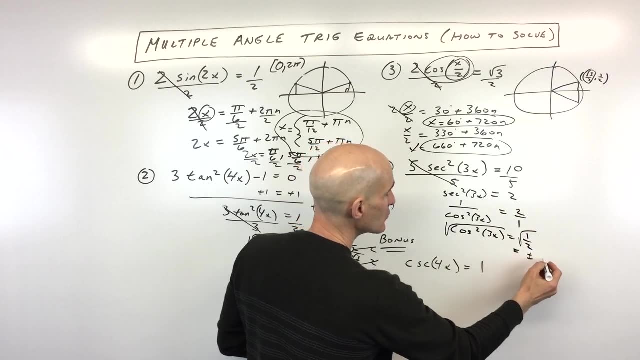 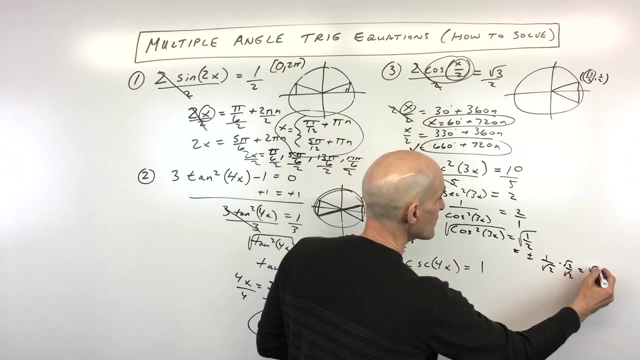 of both sides of this equation. so if i do that, i get: cosine squared of 3x is equal to one-half if i take the square root of both sides, remember you get two answers, plus or minus. square root of 1 is 1, square root of 2. we can rationalize this. this is going to be root 2 over root 2. 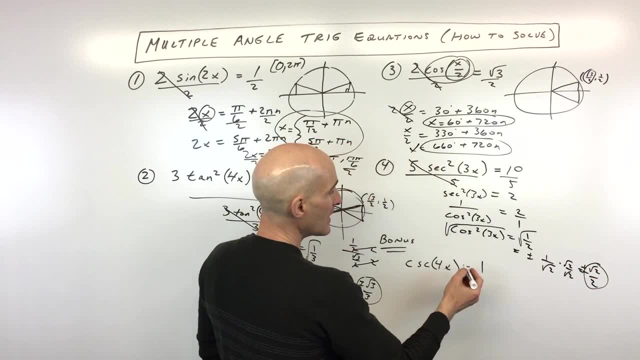 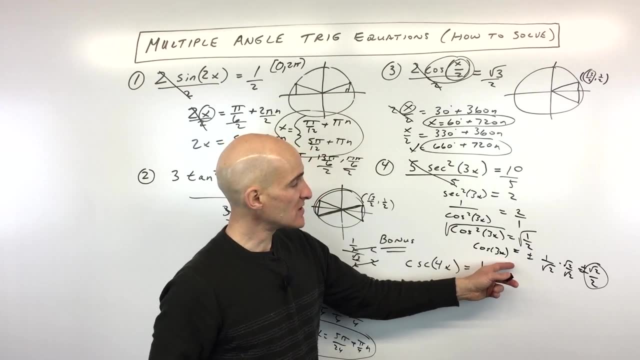 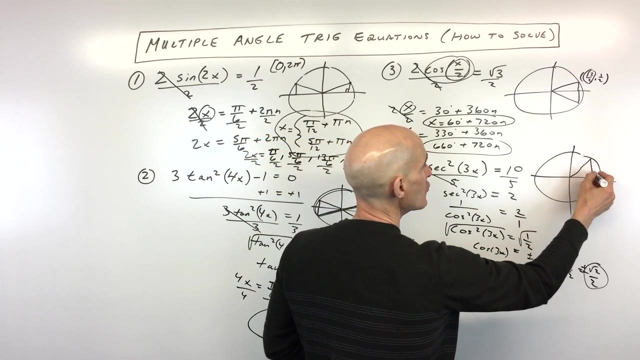 that which is square root, 2 over 2 plus or minus, and so that's saying the cosine of 3x. okay, so now let's go to our unit circle. so where does cosine equal positive or negative root 2 over 2. okay, if we draw our unit circle, cosines the x, it's going to be root 2 over 2 here, negative root 2 over 2. 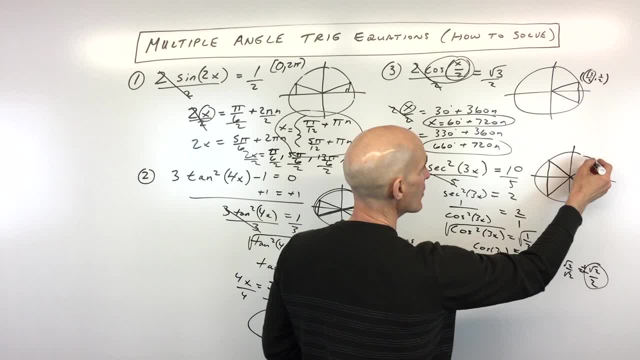 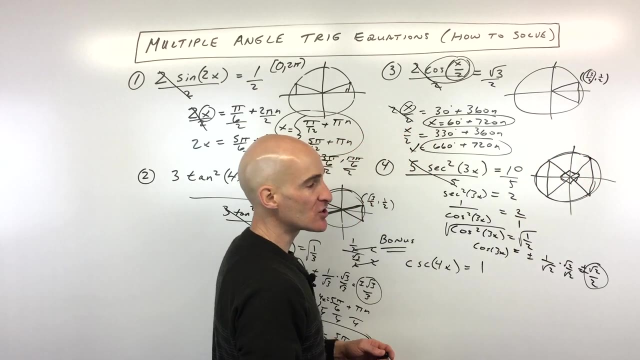 here. negative root 2 over 2 here. positive root 2 over 2 here. but what's interesting about this particular problem is that, see, these are 45 degree reference angles, okay, but notice how these points are actually 90 degrees apart. okay, and so what we can do if we write this as a general, 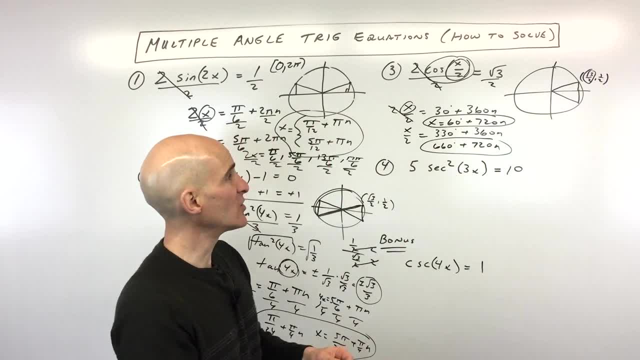 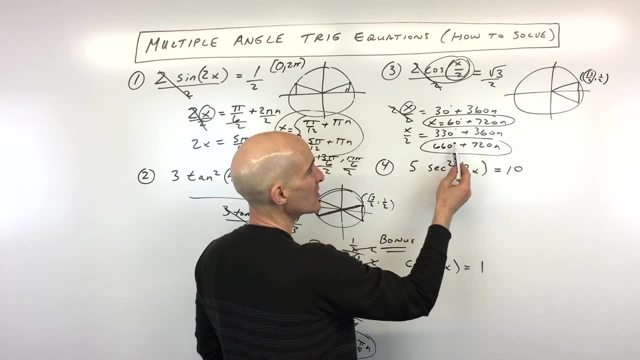 they just said find all the solutions from 0 to 360 meaning you know once around the unit circle here if we let n equals 0 you can see we're getting x equals 60 degrees here if we let n equals 0 we're going to be getting 660 degrees which is not in a restricted domain of 0 to 360 right so you would only just get one solution here just 60 degrees if that was the restricted domain but here if we're writing 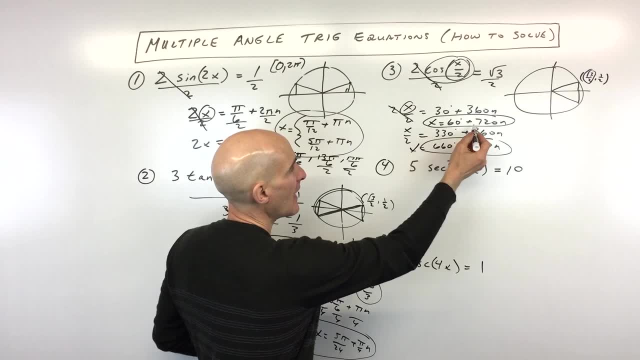 this as a general solution you know we can just have it written as 60 plus 720n or 660 plus 720n 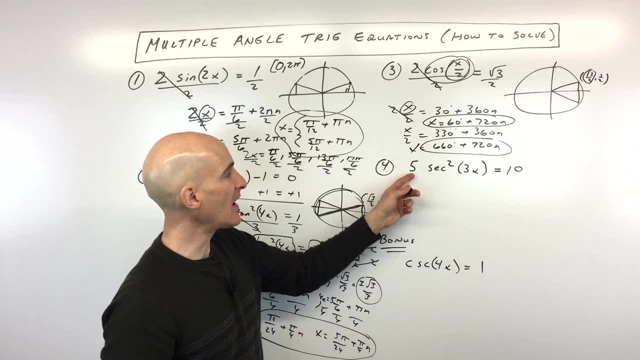 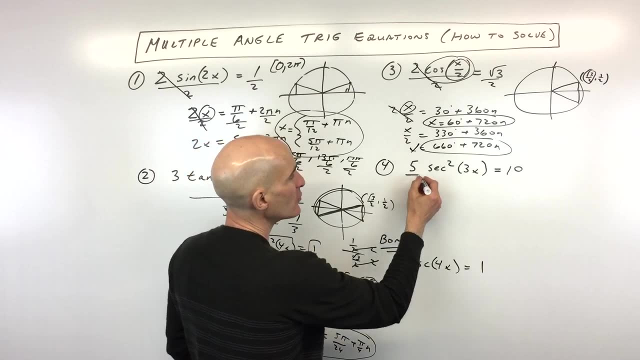 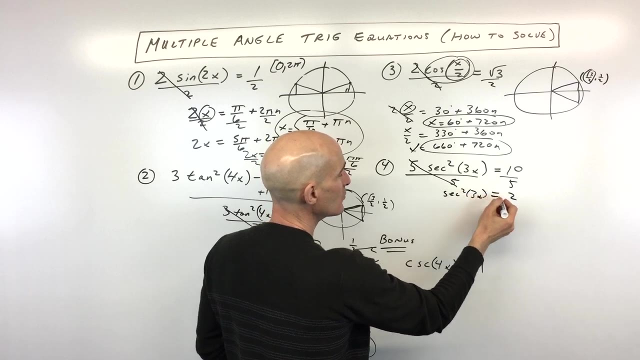 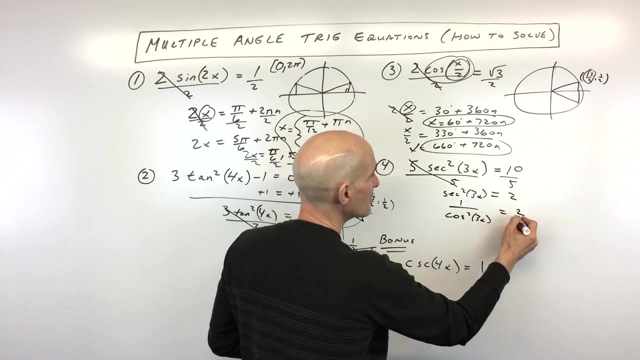 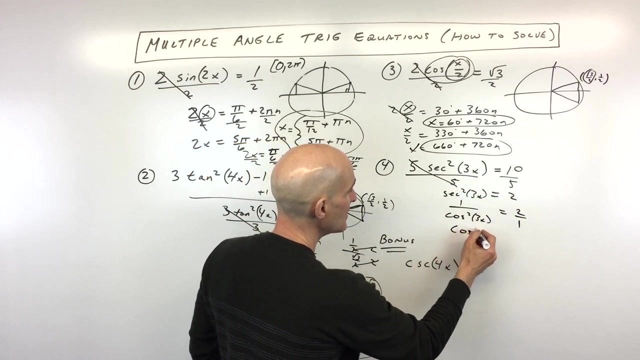 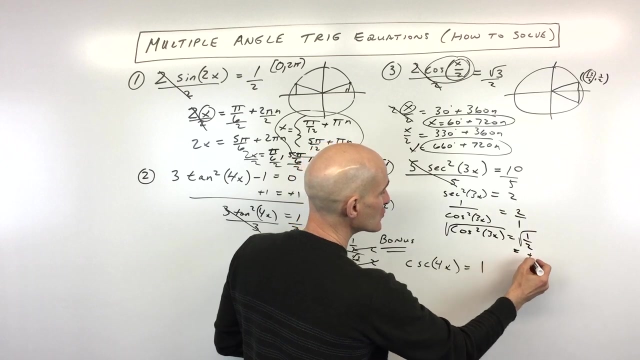 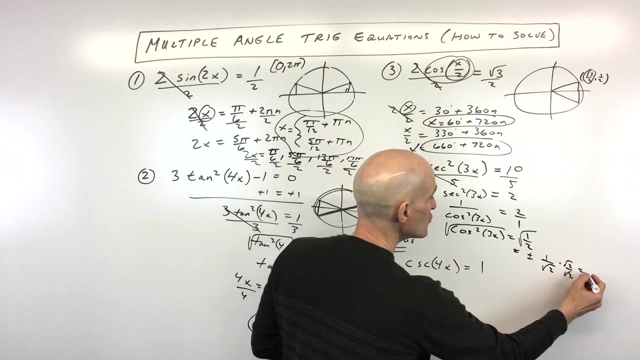 okay let's go on to a fourth example here now so number four we've got 5 secant squared of 3x equals 10 so hmm so how are we going to solve the same idea we're going to divide both sides by 5 we're trying to get that secant by itself so that comes out to 2 so we're saying secant squared of 3x is equal to 2 secant though is really what it's the reciprocal of cosine 2 is like 2 over 1 but now what i'm going to do is i'm going to take the reciprocal of both sides of this equation so if i do that i get cosine squared of 3x is equal to one half if i take the square root of both sides remember you get two answers plus or minus square root of 1 is 1 square root of 2 we can rationalize this this is going to be root 2 over root 2 like that which is square root 2 over 2 plus or minus and so that's saying the cosine of 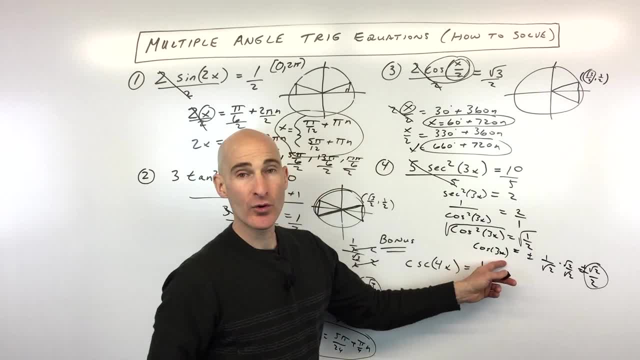 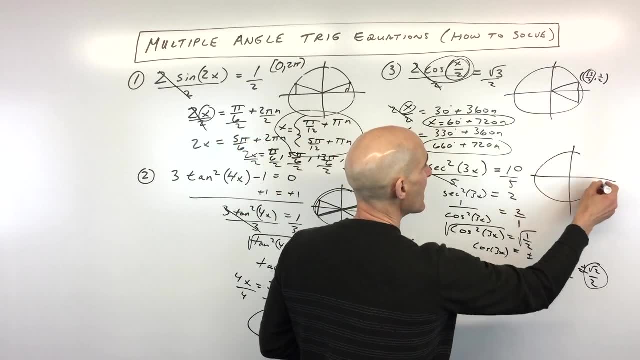 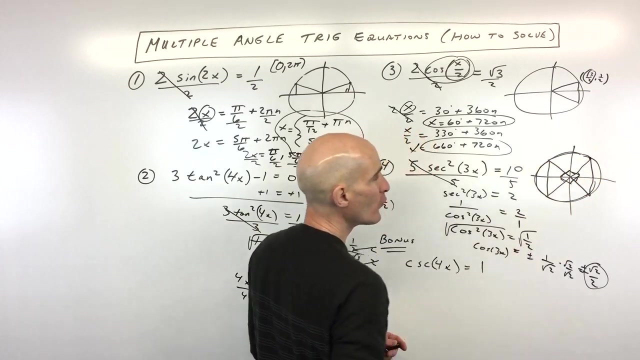 3x okay so now let's go to our unit circle so where does cosine equal positive or negative root 2 over 2 okay if we draw our unit circle cosines the x it's going to be root 2 over 2 here negative root 2 over 2 here negative root 2 over 2 here positive root 2 over 2 here but what's interesting about this particular problem is that see these are 45 degree references angles okay but notice how these points are actually 90 degrees apart okay and so what we can do if we write this as a general solution is we could say 3x equals pi over 4 so 45 degrees 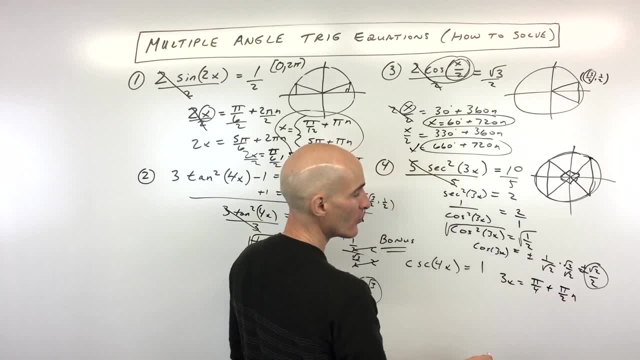 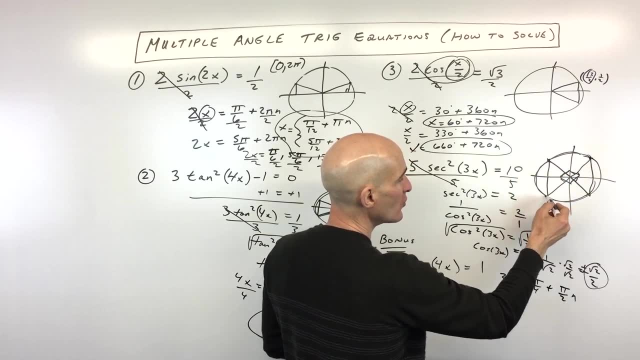 plus 90 degrees or pi over 2 radians times n so what we're doing is we're adding 90 degrees that takes us to the next point where cosine is equal to root 2 over 2 and we keep adding 90 degrees and we keep basically bouncing around to the next corresponding 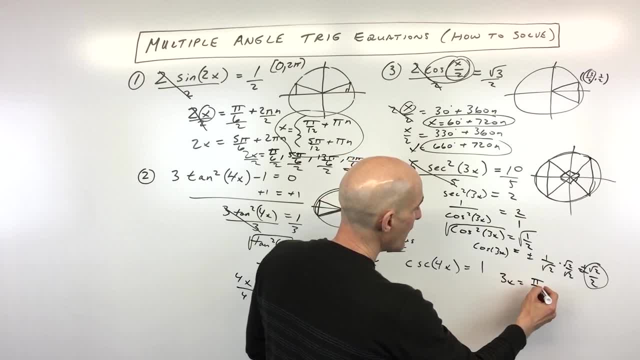 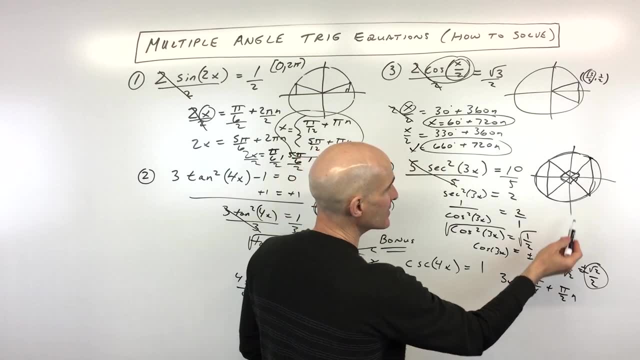 solution is: we could say: 3x equals pi over 4, so 45 degrees plus 90 degrees, or pi over 2 radians times n. so what we're doing is we're adding 90 degrees. that takes us to the next point, where cosine is equal to root 2 over 2, and we keep adding 90. 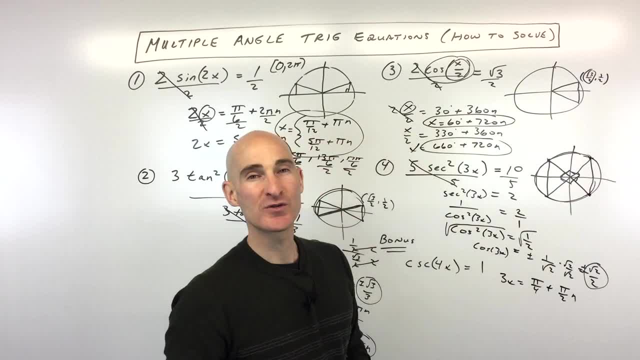 degrees and we keep basically bouncing around to the next corresponding. 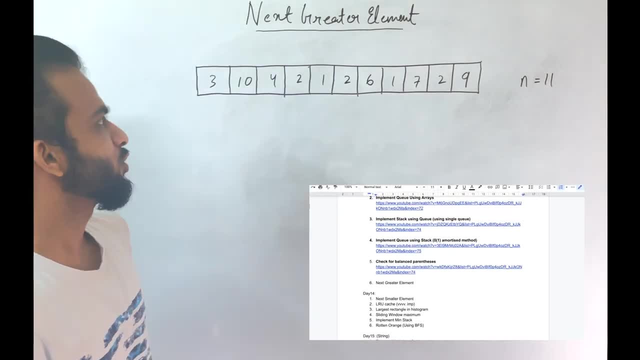 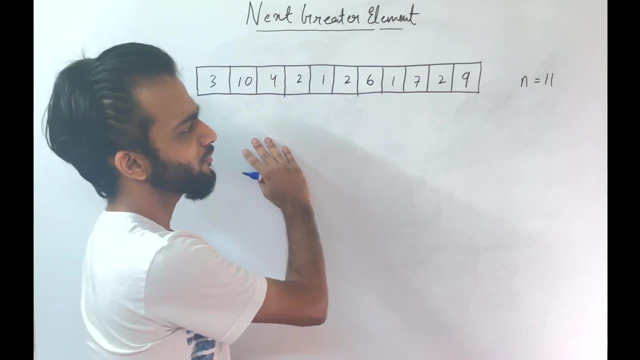 hey, everyone, welcome back to the channel. i hope you guys are doing extremely well. so today we will be solving the problem. next, greater element. what does that state? basically, you will be given an array of n elements. over here i have taken an 11 size array. you have to. 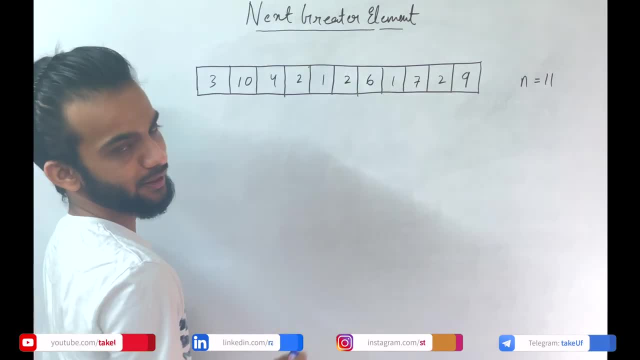 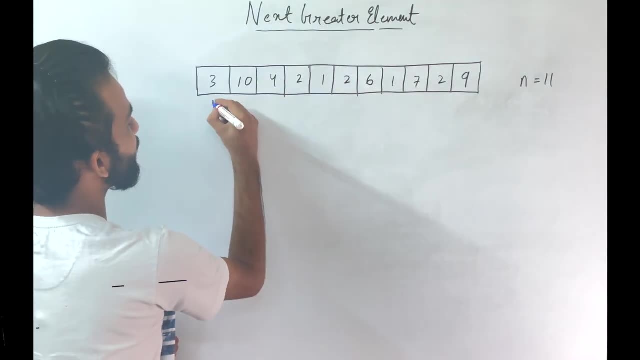 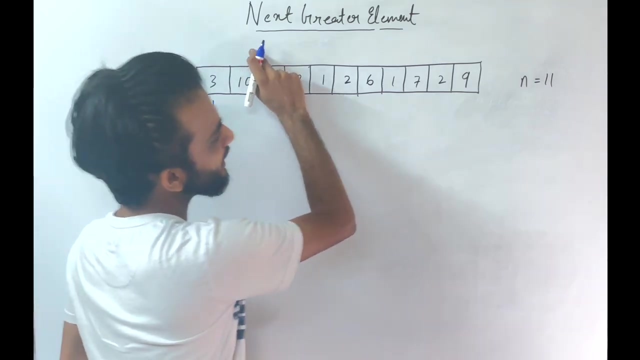 figure out for every element which is the next greater element. okay, for an example, if you stand at 3 and you look at the right, the next greater element that you will get for 3 is nothing but 10, because 3 upon 3, the next greater element is 10.. now, if you stand at 10 and you look at the, 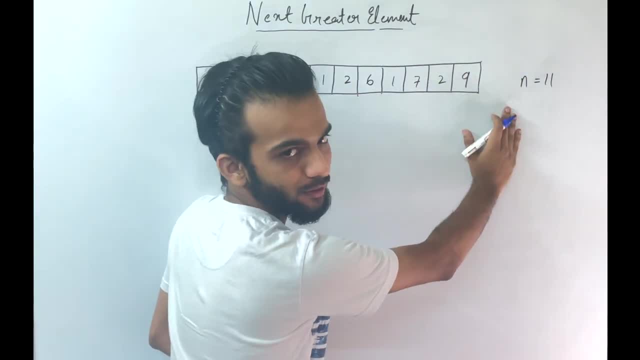 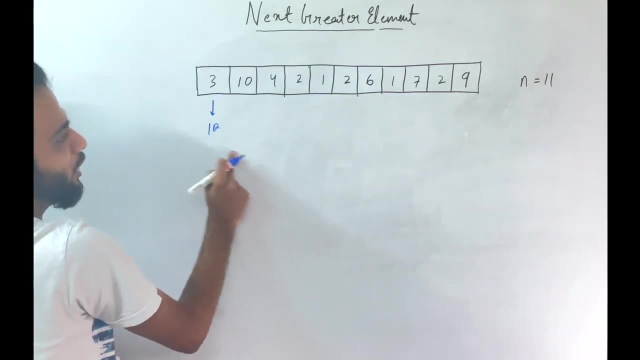 right, you will not see anyone greater than 10. okay, you will not see anyone greater than 10. and if you do not see anyone greater than 10 on the right, you will come back and look across here. do you see anyone from this side? first you look across this side. you don't find anyone. then you start looking. 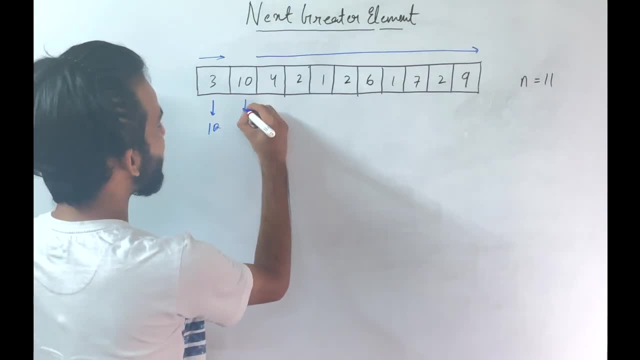 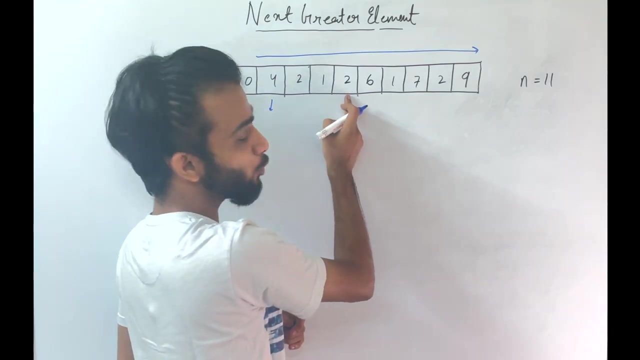 from this side. do you find anyone? you don't. so if you do not find anyone, you just write minus 1 and not 8, because there are no right answers from 16 and 11, you will be going right across here. do you find anyone from this side? first, you will come back and look across here. do you find? 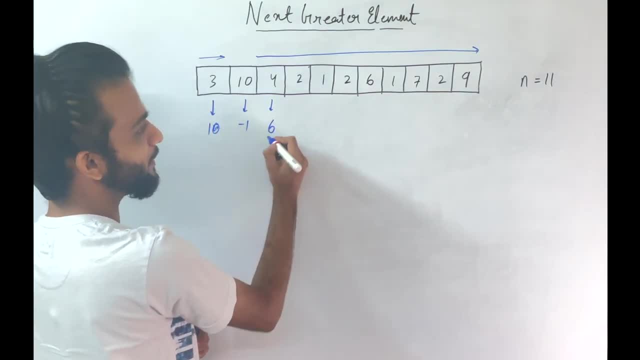 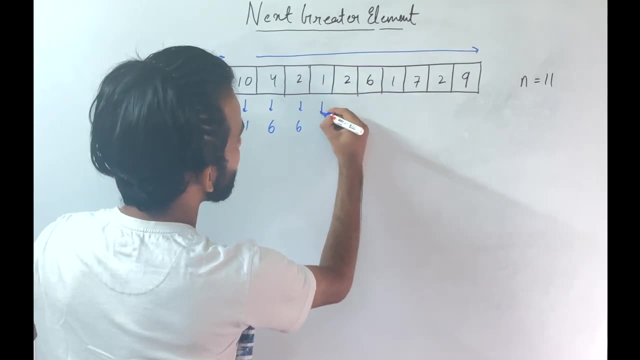 anyone over here, and you will never see anyone that is greater than 10, because 0 is the first greater element. then you will find a last, fully greater element, so do not forget your subtraction: no, number ten, Вас is alsoняя number one, because there is no next greater element, and straight for.